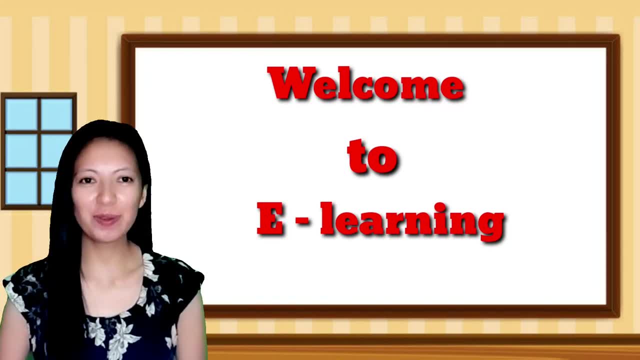 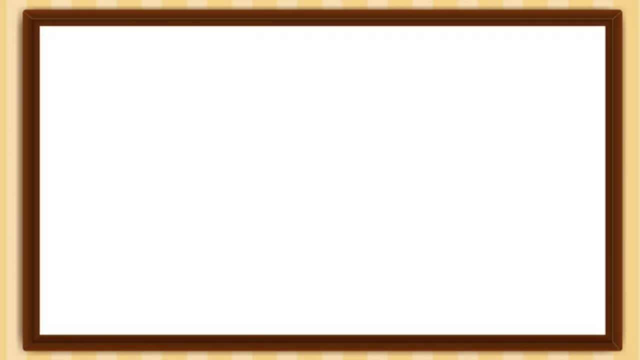 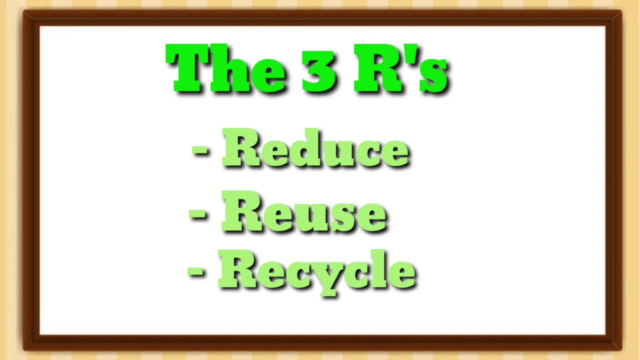 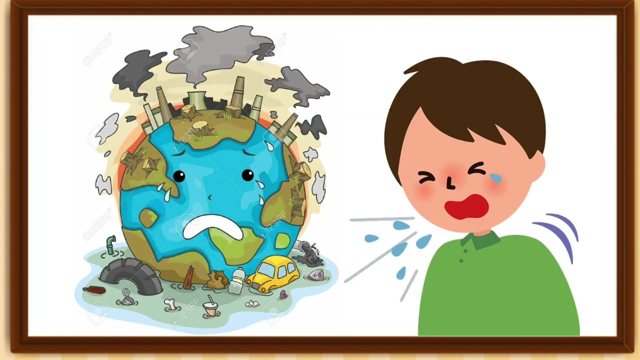 Hello guys, this is Teacher Louie. Here's another new video for you. Hope you enjoy. Today's topic is about the three R's: Reduce, Reuse and Recycle. Are you tired of cleaning your trash every day? Are you feeling sick because of pollution? 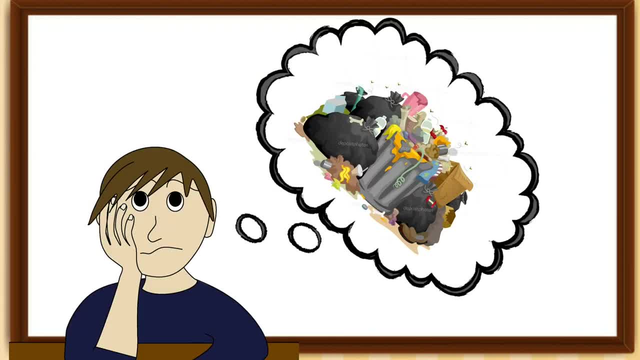 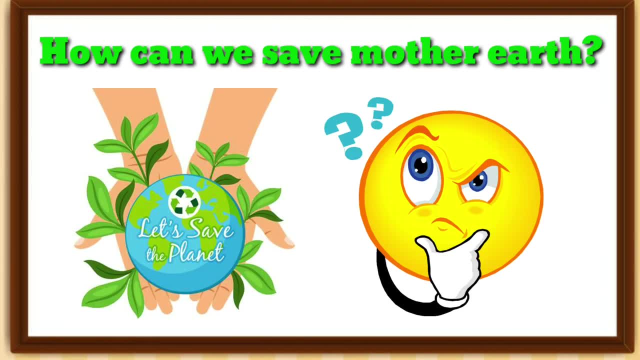 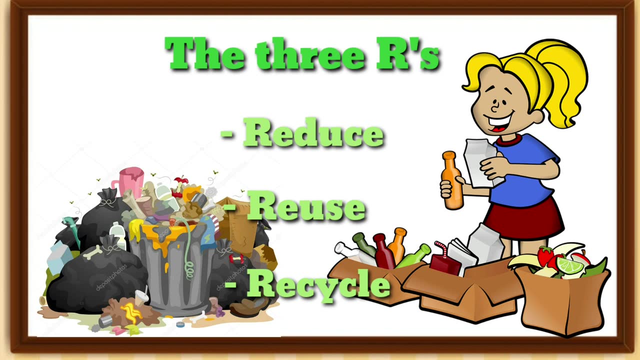 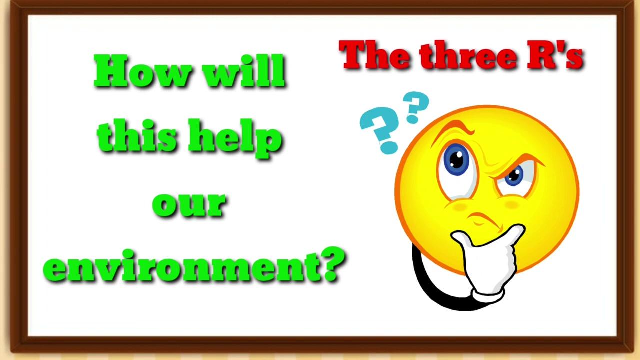 Are you worried about the environment? How can we save Mother Earth? The three R's- Reduce, Reuse and Recycle- can help decrease the amount of garbage we produce. How will this help our environment? The first R stands for Reduce. 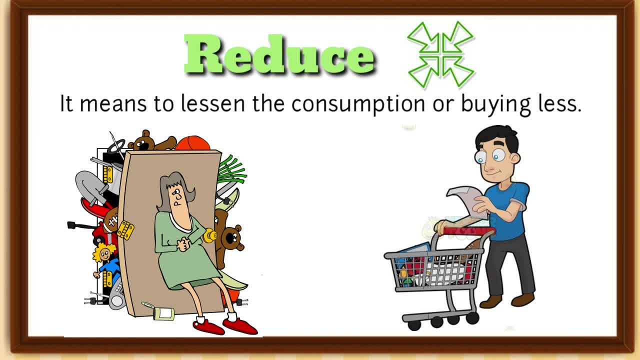 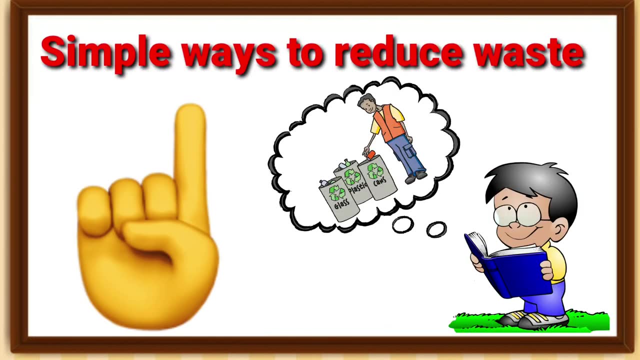 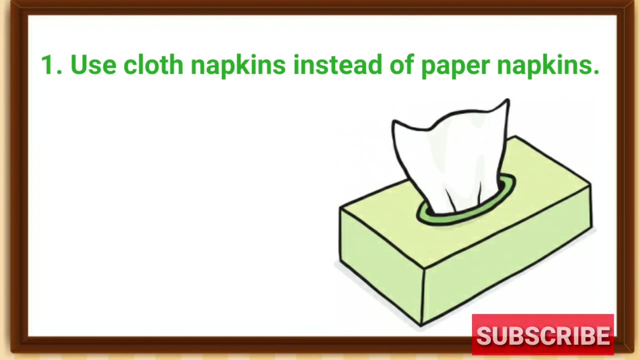 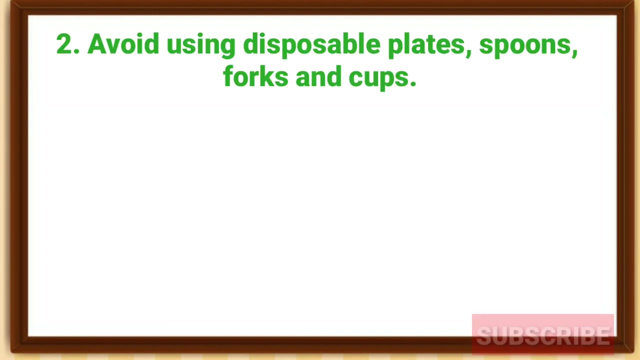 It means to lessen the consumption or buying less. If there is less waste, then there is less to recycle or reuse. Here are the simple ways on how to reduce our waste: Use cloth napkins instead of paper napkins. Avoid using disposable plates, spoons, forks and cups. 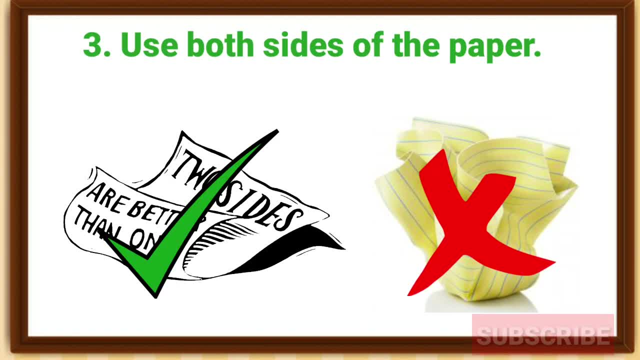 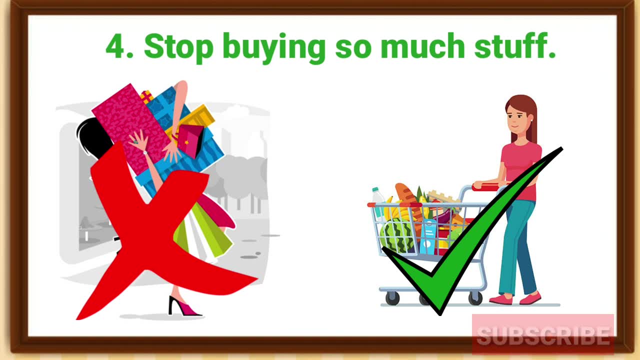 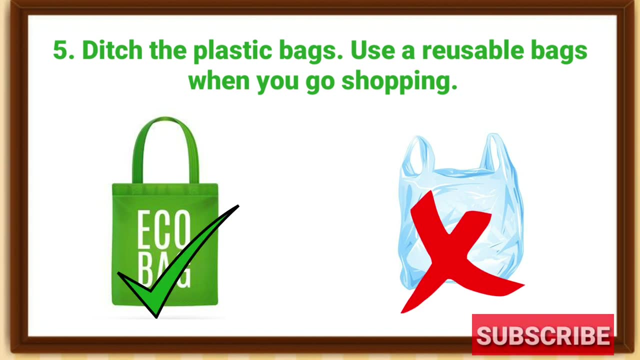 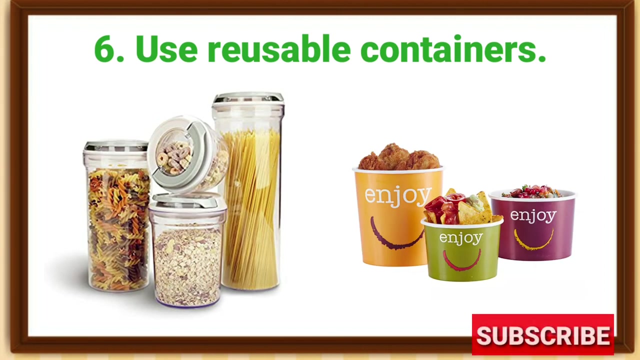 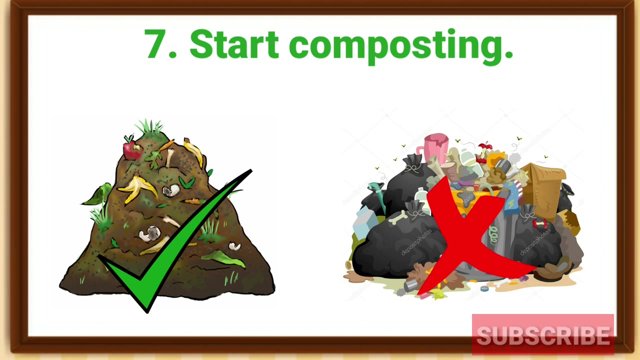 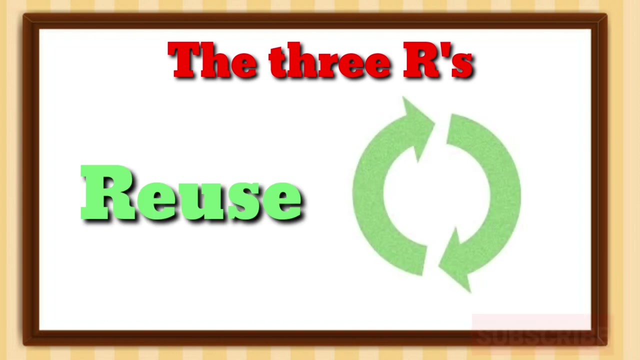 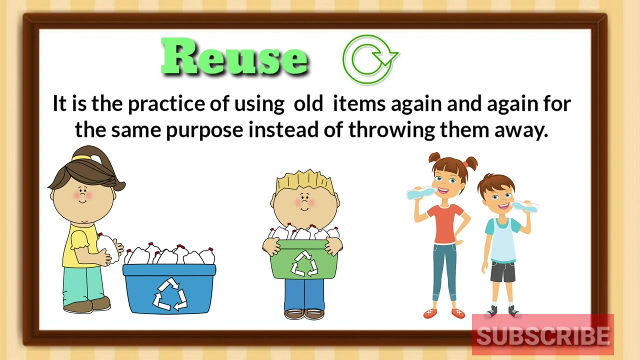 Use both sides of the paper. Stop buying so much stuff. Ditch the plastic bags. Use a reusable bag when you go shopping, Use reusable containers And start composting. The second R stands for Reuse. It is the practice of using old items again and again for the same purpose, instead of throwing them away. 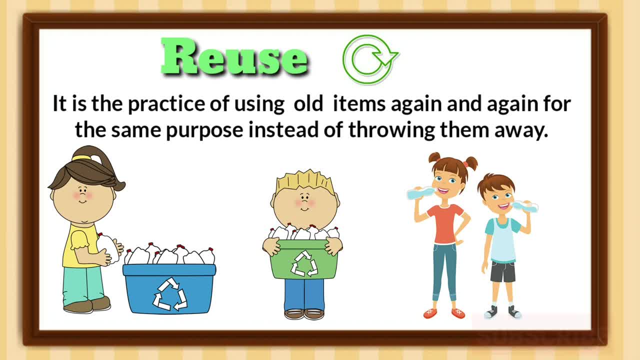 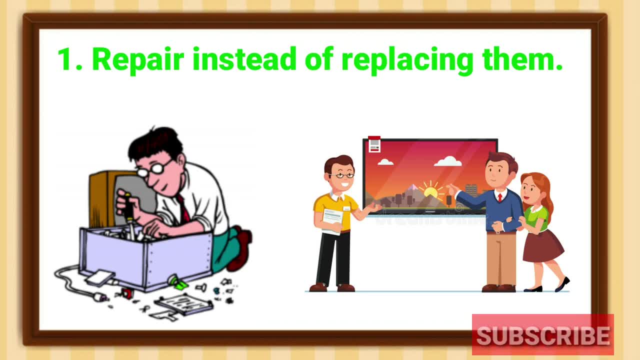 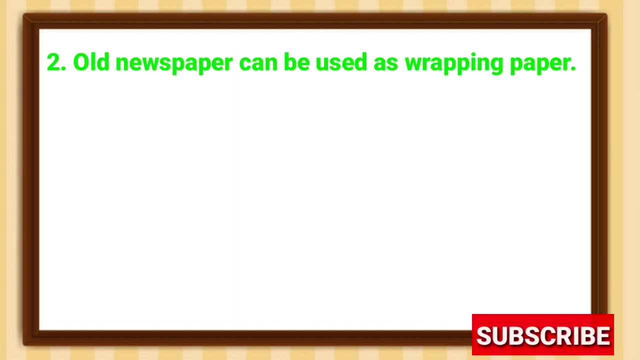 Stacking them into a glass container for the waste is better. Here are some ways to reuse items. Coat your heart with good onions. first, Repair items instead of replacing them in a greenhouse. Put a lid on the windows to prevent the them from spreading. 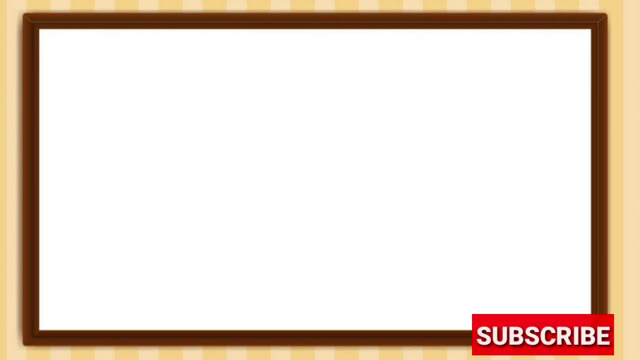 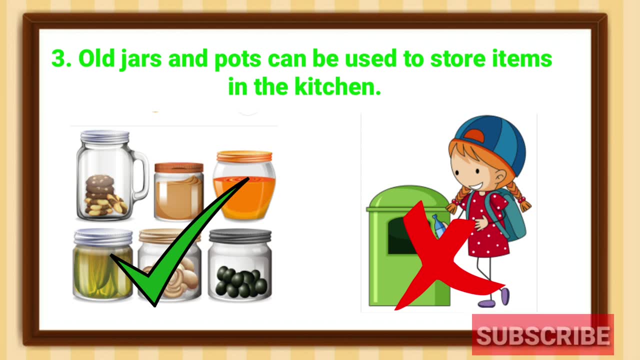 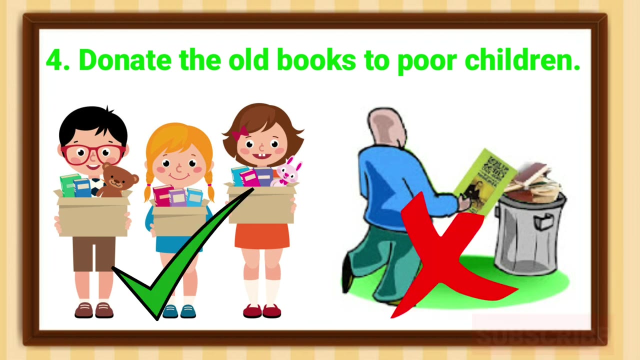 On your fridge. if you keep your newspapers like that and the нач A upper with paper can cause aiverso in your ل format that I might be solve it later. store items in the kitchen. Donate the old books to poor children, Old clothes. 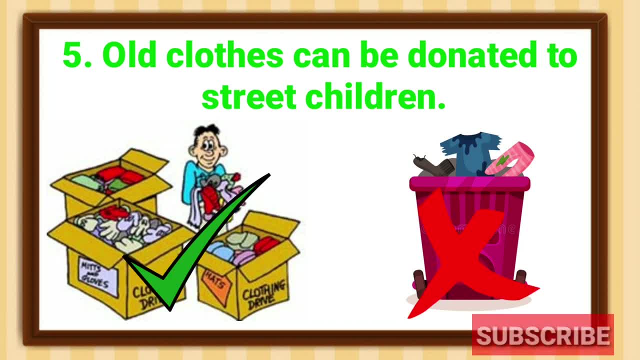 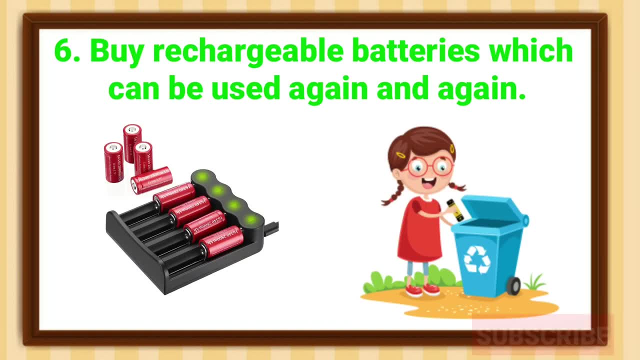 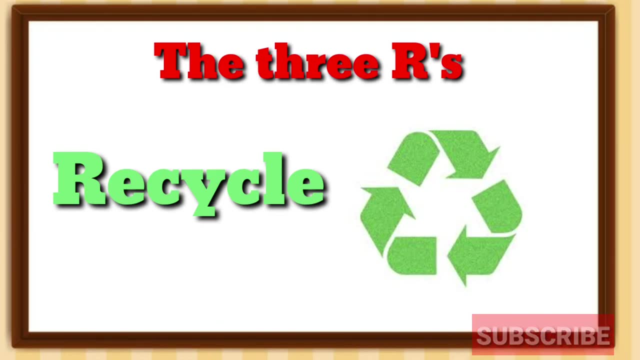 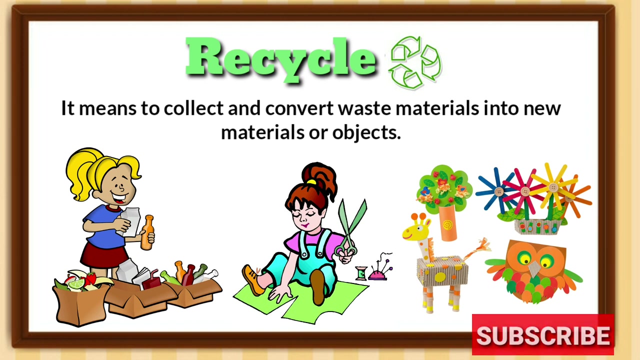 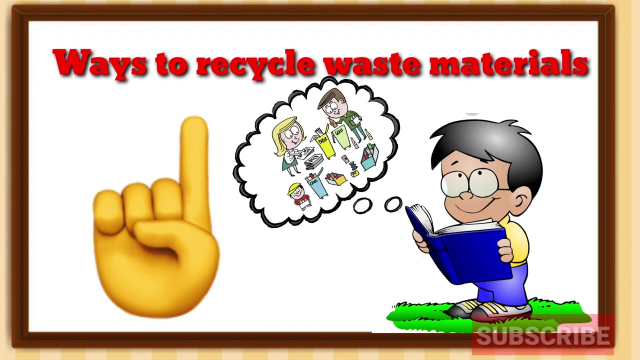 can be donated to street children. Buy rechargeable batteries which can be used again and again. The third R stands for recycle. It means to collect and convert waste materials into new materials or objects. Here are some ways on how to recycle waste materials. Provide recycling bins. 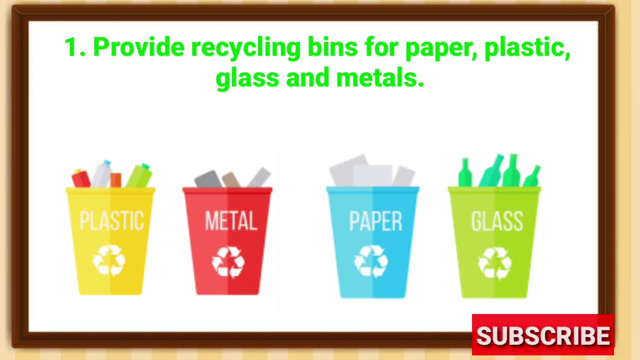 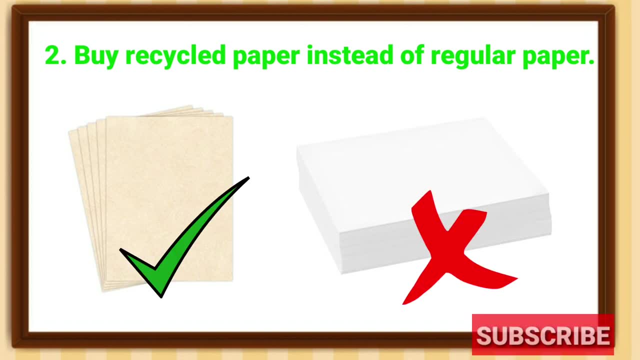 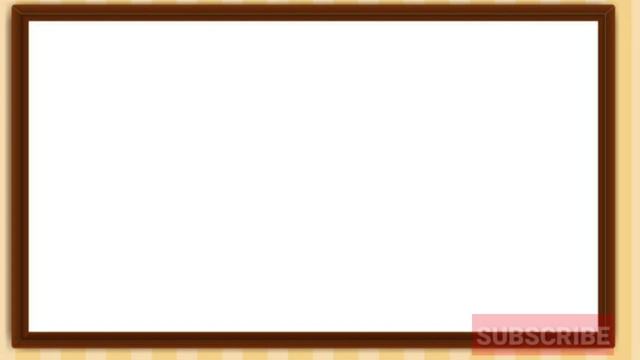 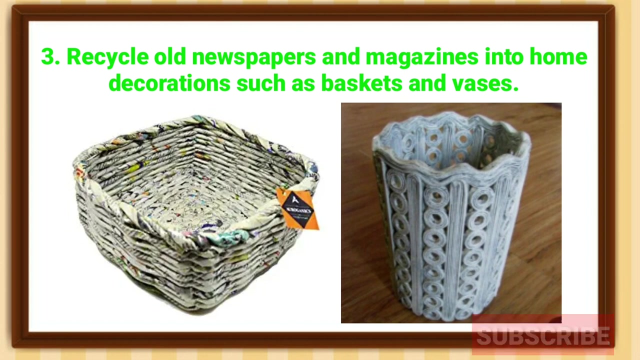 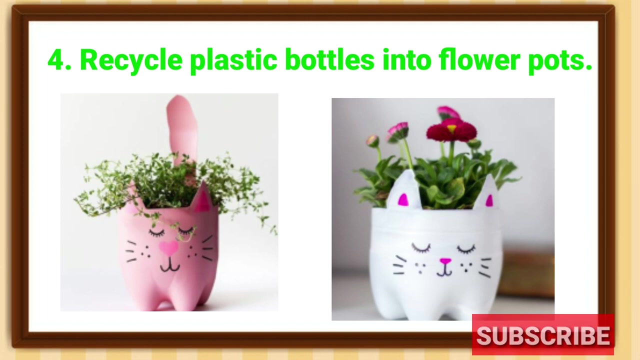 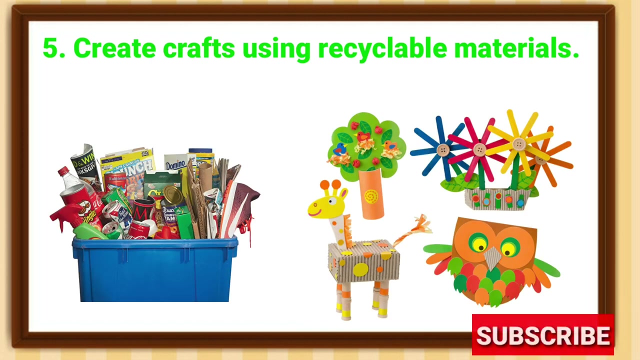 for paper, plastic, glass and metals. Buy recycled paper instead of regular paper. Recycle old newspapers and magazines into home decorations such as baskets and vases. Recycle plastic bottles into flower pots. Create crafts using recyclable materials. What materials can and can't be recycled? 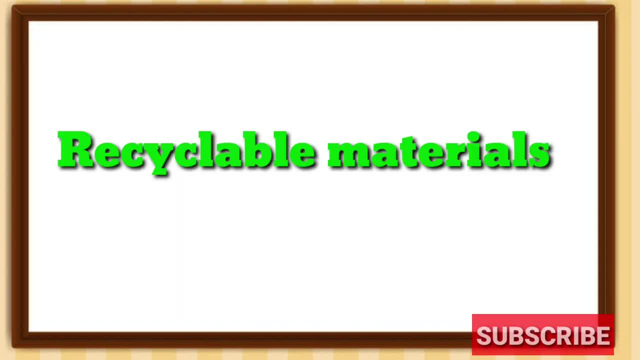 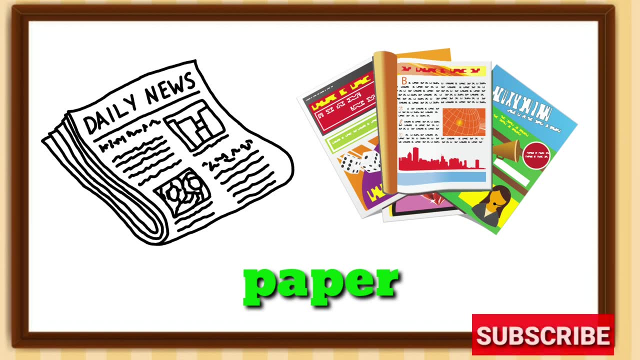 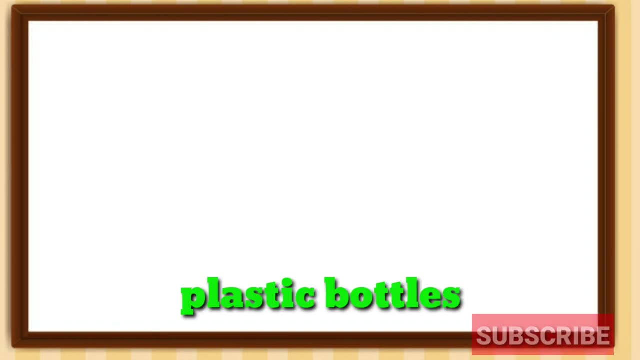 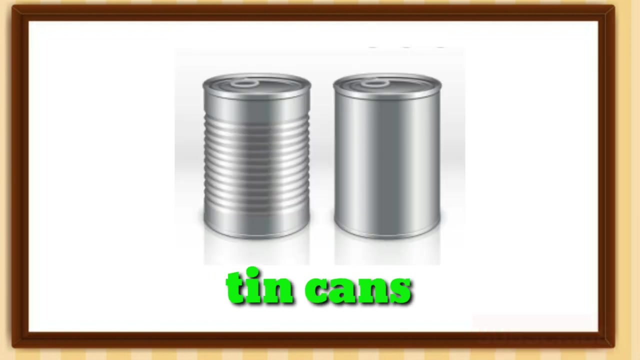 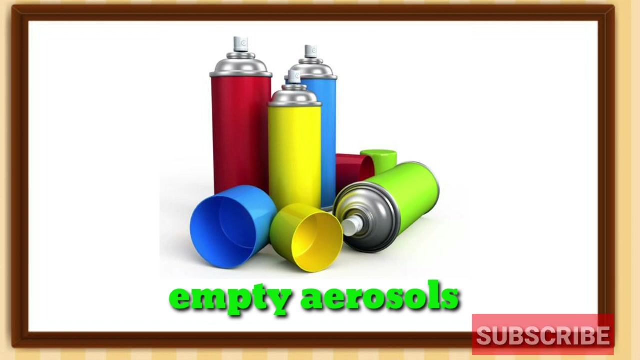 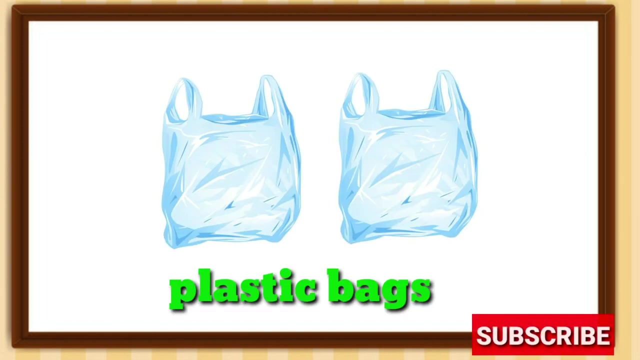 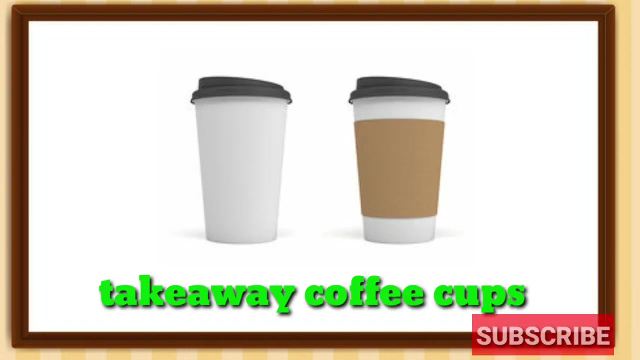 The following are the materials that we can recycle: Paper, Cardboard, Cartoons, Plastic bottles, Clear bottles, Tin cans, Jars, Empty aerosols. The following are non-recyclable materials: Plastic bags, Takeaway coffee cups, Disposable nappies, Polystyrene Bubble wrap.